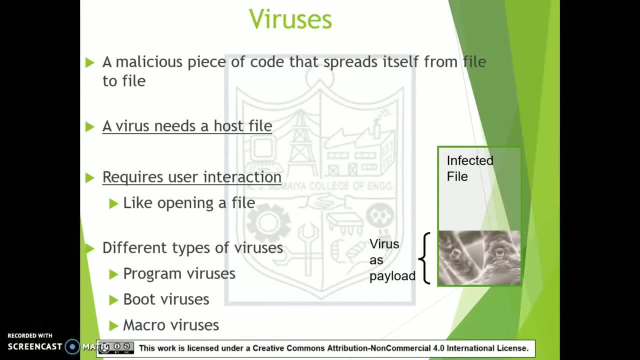 unknown email which contains a virus, then your your computer will be affected by the virus. So we have to be very careful while opening an unknown file or unknown email and we have to look for an antivirus software first that it is not affected by the virus. Now, different kind of 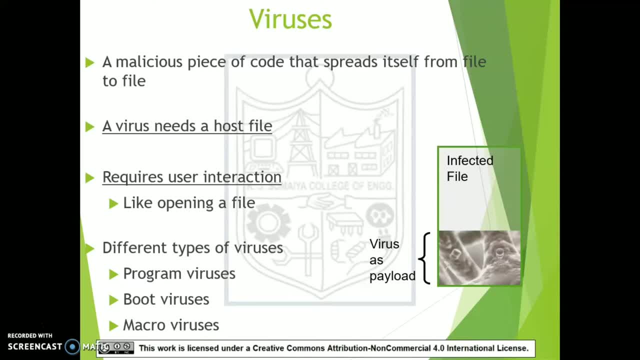 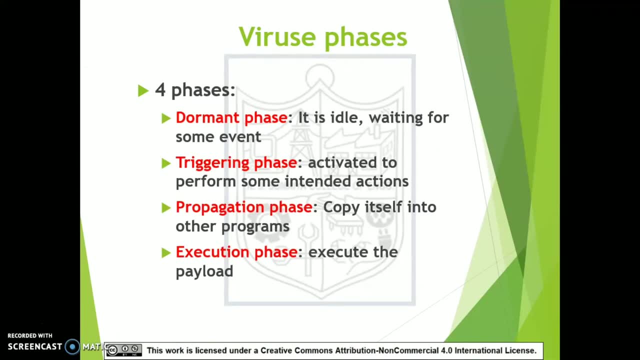 viruses which are going to discuss here is program viruses, boot viruses and macro viruses. Now there are four phases of viruses: Dormant phase, triggering phase, propagating phase, propagation phase and execution phase. So what happens in the dormant phase? At dormant phase the virus is idle and not doing anything. At triggering, 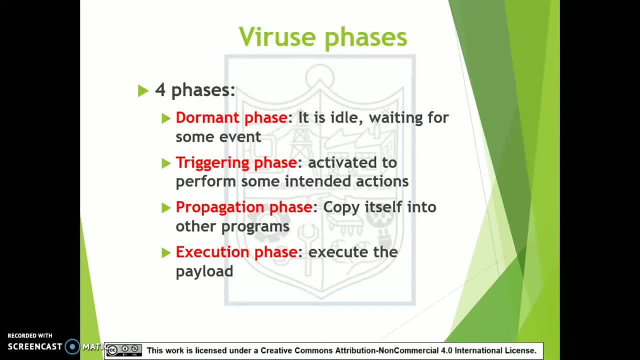 phase, the virus is activated to perform the function for which it was intended. As with the dormant phase, the triggering phase can be caused by a variety of systems or events, including the count of numbers or times. the copy of the virus has made copies of itself. What happens at a propagation phase? At propagation, 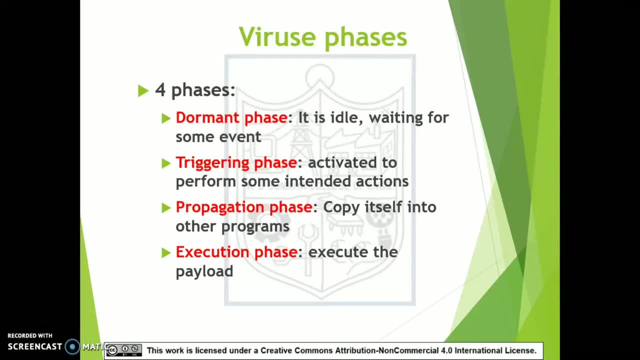 phase, the virus is activated, It starts to replicate itself into other programs. Now this is a propagation phase and at finally, execution phase. At propagation phase, the virus has been triggered, The payload is obviously executed. This could have been harmful and damaging, such as displaying text to the user, spamming. 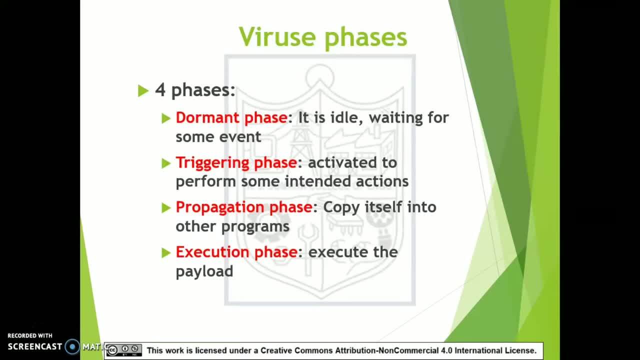 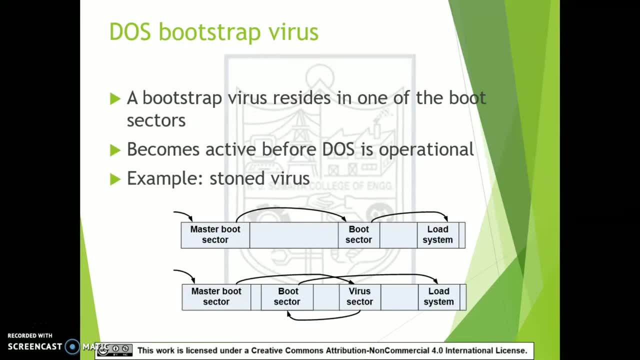 the network, destroying the hard drive. you name it. you can anything that the virus can do to execute it. This is the execution phase. Now, what is Doge bootstrap virus? A bootstrap virus resides in one of the boot sector. The infected code runs when the system is booted from an infected disk. 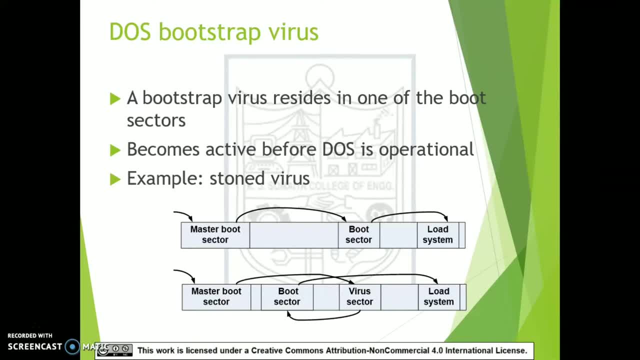 but once the loaded, it will infect other floppy disks. It is affected mostly by the floppy disks which is outdated right now, but this was the main reason for which the floppy disks has been outdated- from the computers. The example of this kind of virus is stoned. 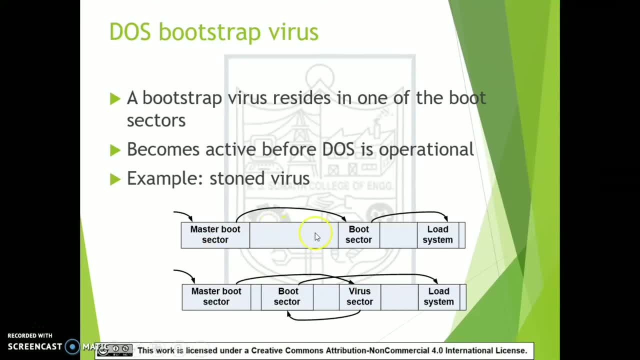 virus. Here we can see the master boot sector, where no virus is affected, and here the computer which is affected by the virus, where virus sector is also been booted when the computer is booting or starting. so this is the bootstrap virus. now, what is parasitic virus? parasitic. 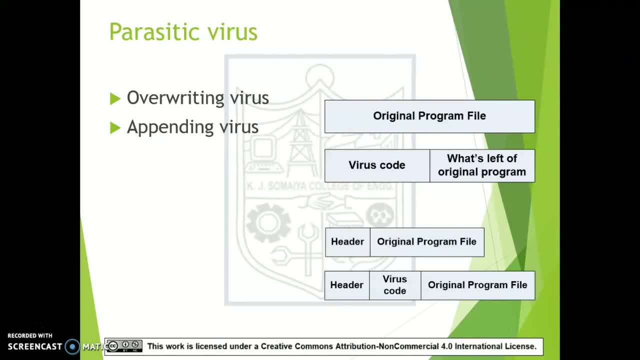 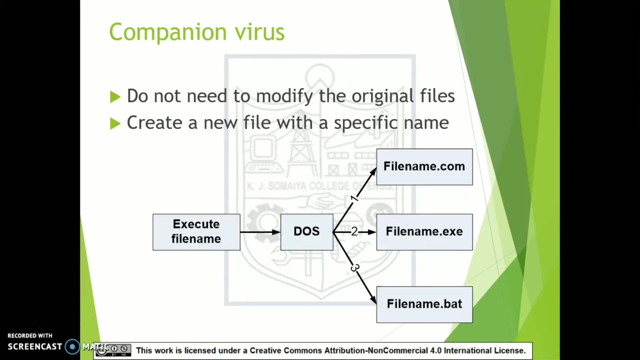 virus is attached themselves to programs. hence a user launches a program that has a parasitic virus, the virus serpentiously is launched first now to cloak its presence from the user. the virus then triggers the original program to open the same virus. now companion virus. a companion virus generally do not 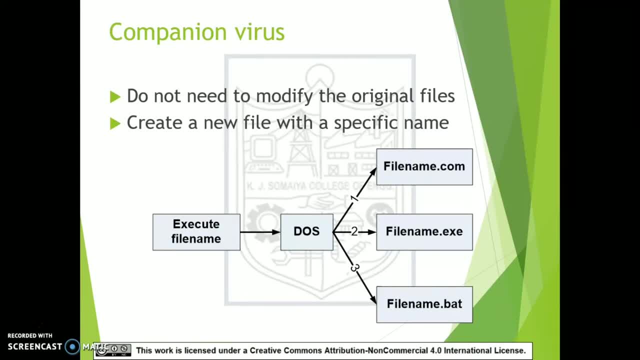 need to modify the original files. they are. they are done with the same file or the same file name which is stored in the computer. our companion virus is a computer virus that stores itself in a file that is named similar to another program file that is commonly executed. when that file is executed, the virus will infect. 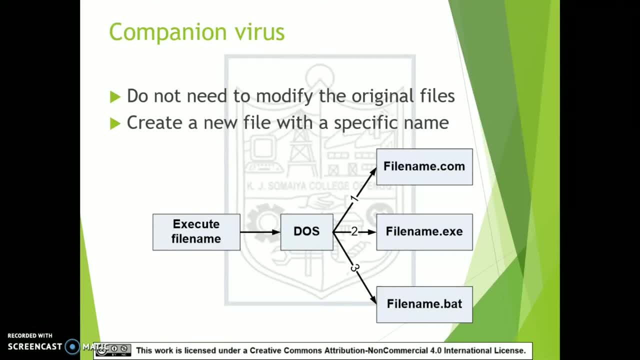 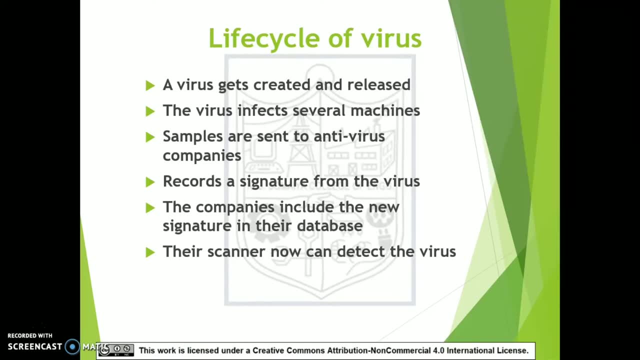 the computer or perform malicious steps such as deleting the files on your computer or hard drive. life cycle of a virus. a virus gets created and released. the virus infects several machines and it gets affected thoroughly by the machines. now, once the virus becomes very common and has affected many of the common computers, it goes. 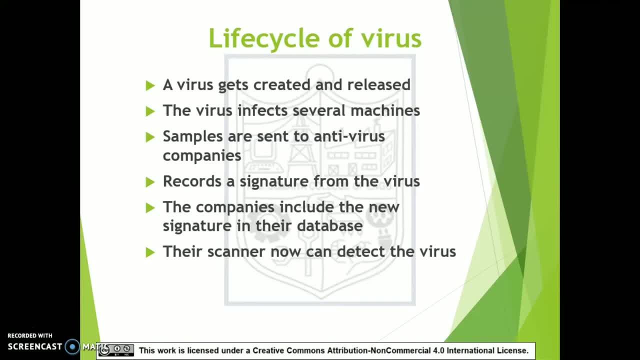 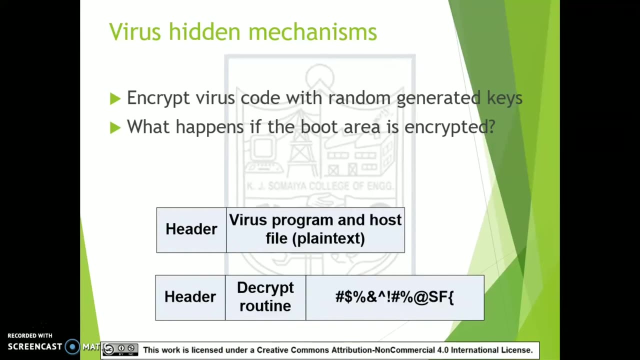 into the antivirus companies. they record the signature of the virus and the companies include the new signature in the database, which can easily detect the virus and can combat it. now what is the mechanism of virus? normally, virus encrypt the data by using random generated keys and can encrypt your computer data. 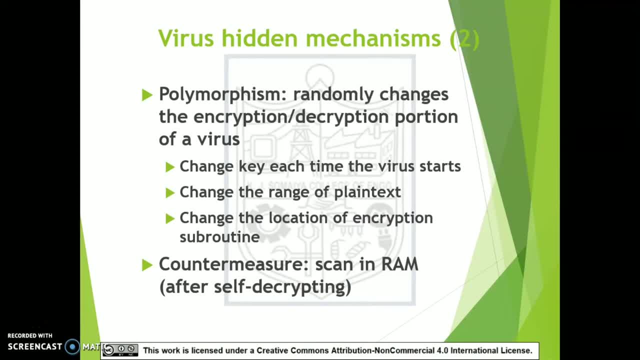 now polymorphism. what is polymorphism? the most recent class of viruses to appear on the screen are the polymorphic or self-mutating viruses. these are the viruses that infect their targets with the modified or encrypted versions of themselves. now by varying the code sequence written to the file or by generating a different random encryption key. 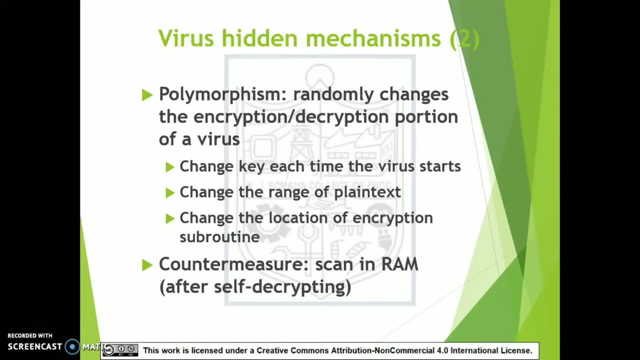 the virus is altered, file will not be identifiable, though the use of simple by matching to detect the presence of these viruses requires that a more complex algorithm been employed. in effect, this reverses the masking to determine if the virus is present or not. they normally change the key each time the virus starts. they change the range of the plane tags, change the location of the 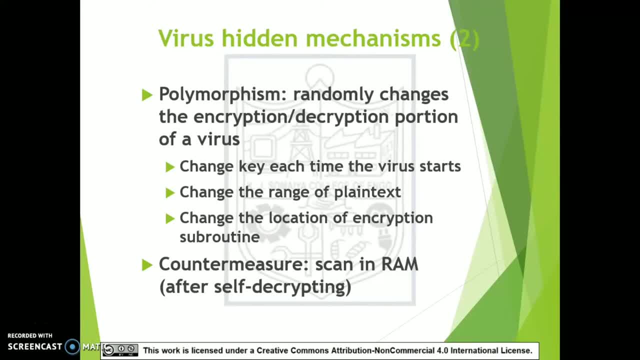 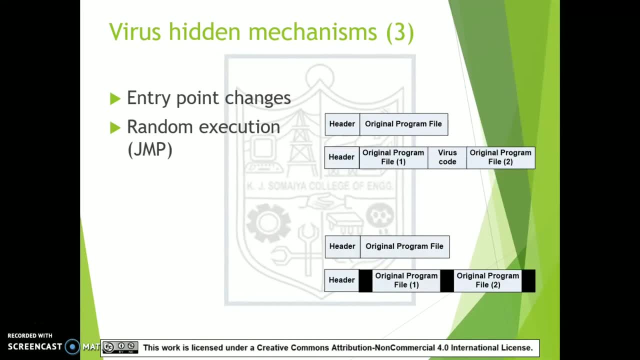 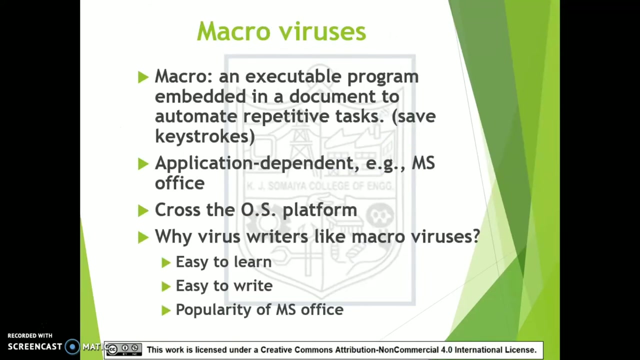 encryption subroutine. these are the polymorphism or polymorphic viruses entry point and this is the header file of a virus. the header position normally replaces the original file program and can run on that file program. now, what are macro viruses? macro viruses are short snippets of code written in a language which is typically interpreted by the application. 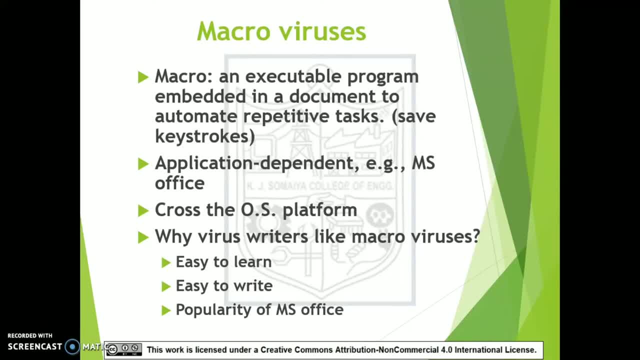 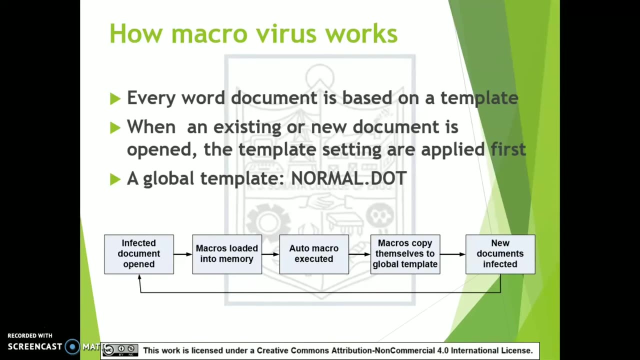 uh, an executable program embedded in the document. automate repetitive tasks, application dependent, like ms office. why virus uh virus writers, like micro viruses? because this is easy to learn, easy to write, popularity of ms office. every word document is based on template. when an existing or new document is opened, the template setting and applied first. so uh, these. 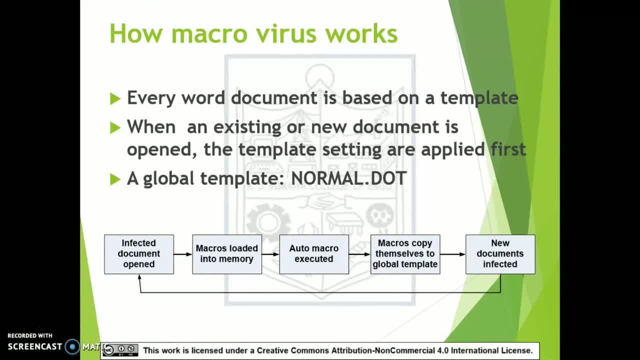 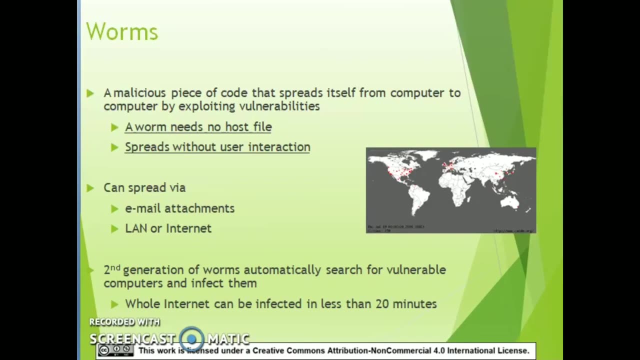 are the viruses that normally affect your computer. this is the life cycle of a micro virus. uh, now my friend Kushal Trivedi will elaborate something on worms and other things. thank you very much. okay, so now, what is worms? a malicious piece of code that spreads itself from computer to computer. 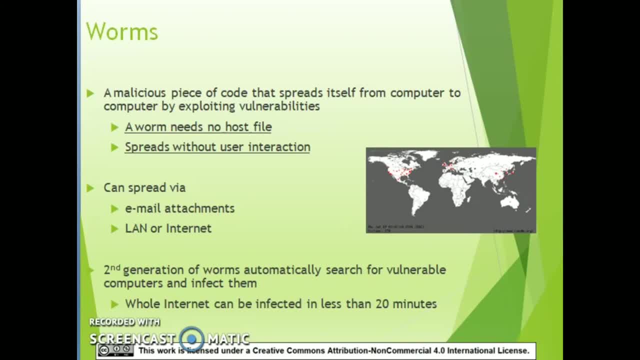 by exploiting vulnerabilities. a worm needs no host file. spreads without user interaction. it can spread via email attachments, lan or internet. the second generation of worms automatically search for vulnerable computers and infect them. whole internet can be infected in less than 20 minutes. worm self-replicating over networks, but not infecting program. 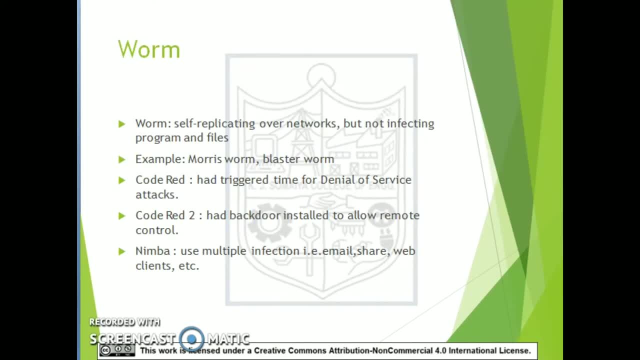 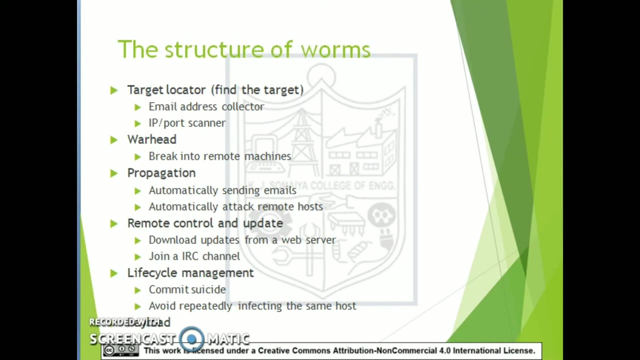 and files. example: Morris worm blast over codered had triggered time for denial of service attacks. code red 2 had backdoor installed to allow remote control. nimba use multiple infection, that is, email, share, web clients, etc. the structure of worms: target locator, email address, collector and ip. 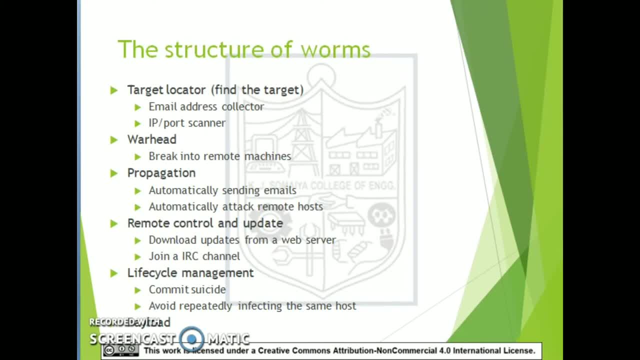 port scanner. warhead breaks into remote mode machines: propagation, automatically sending emails, automatically attack remote host, remote control and update downloads. update from a web server. join our IRC channel. life cycle management commits suicide. avoid repeatedly infecting the same host payload. now what is a worm warhead? a piece of code. 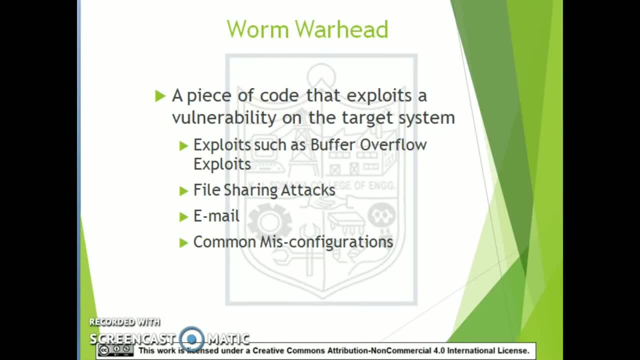 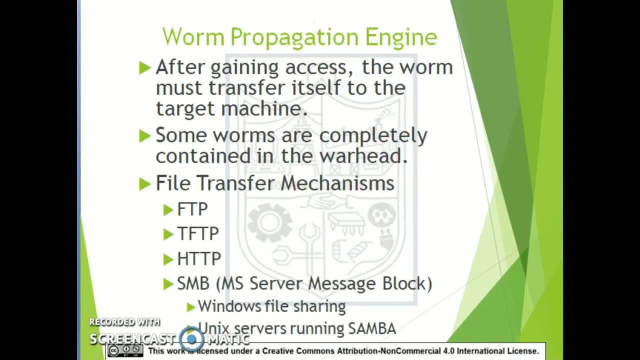 that exploits a vulnerability on the target system. experts, such as buffer overflow exploits, file sharing attacks, email, common mist configuration engine. after gaining access, worm must transfer itself to the target machine. some worms are completely contained in the warhead file transfer mechanisms, such as ftp, tftp, http, smb, ms server. 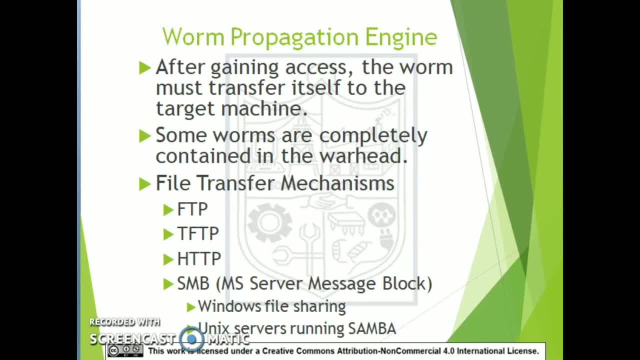 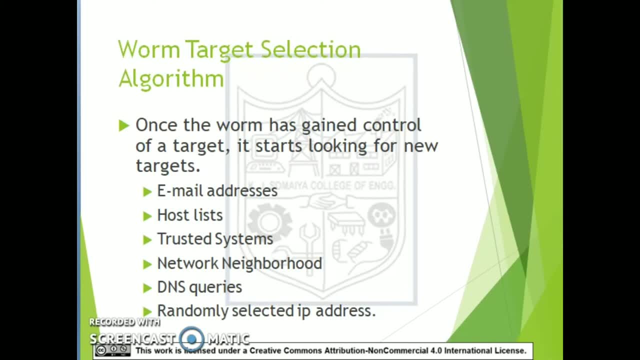 message: block windows file sharing. unique servers running samba worm target selection algorithm. once the worm has gained control over target, it starts looking for a new targets: email addresses, host list, trusted systems, network, neighborhood dns queries, randomly selected ip address worm payload. some specific action done on behalf of the attacker? 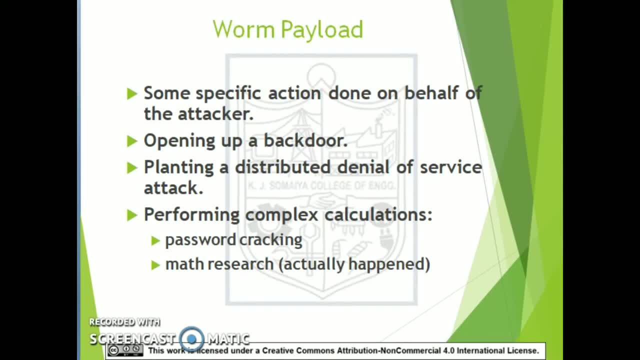 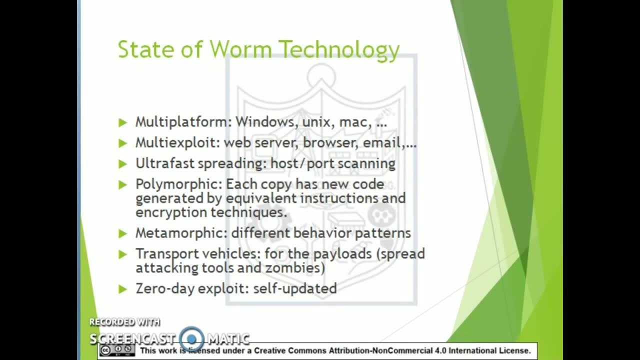 opening up a backdoor, planting a distributed denial of service attack, performing complex calculations, such as password cracking method. research actually happened. there are various state of worm technology, such as multi-platform, such as windows, unix, mac, multi-expert web server, browser, email, ultra fast spreading host or port scanning. 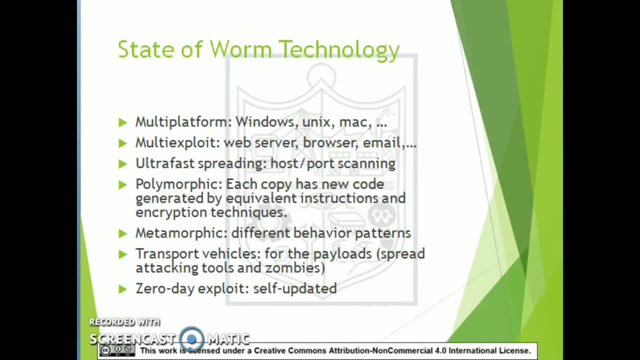 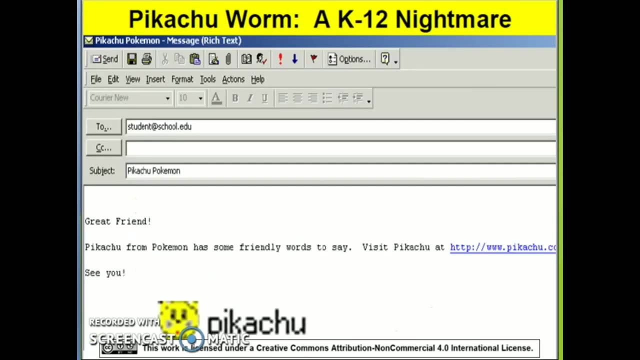 polymorphic: each copy has a new code generated by equivalent instructions and encryption techniques. metamorphic: different behavior patterns, transport vehicles for the payload spread attacking tools and zombie zero-day expert- self-operated. now let's take a look at the pikachu worm, aka 12 nightmare. 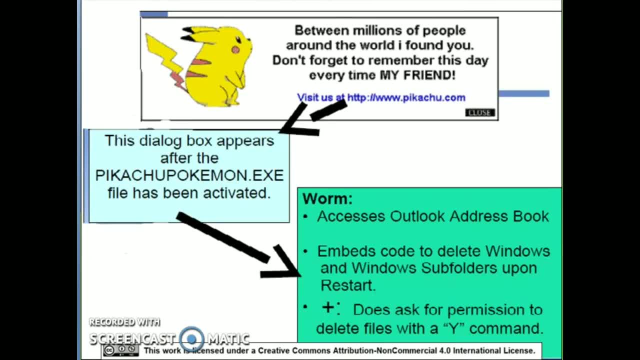 after the mail is sent, the worm gets activated and the dialog box appears as soon as the pikachu pokemonexe file has been activated. what does the worm do? accesses outlook address book, embeds code to delete windows and windows subfolders. upon restart, it does ask for permission to delete files with a y command. now what is the? 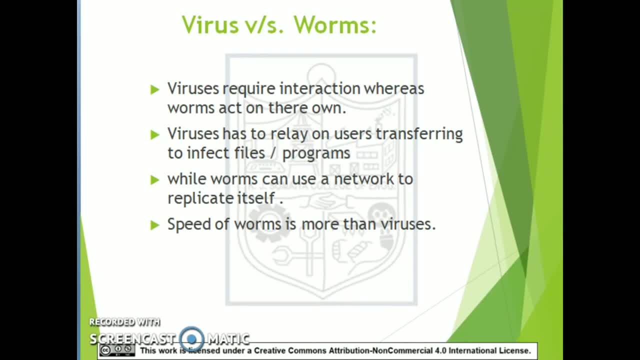 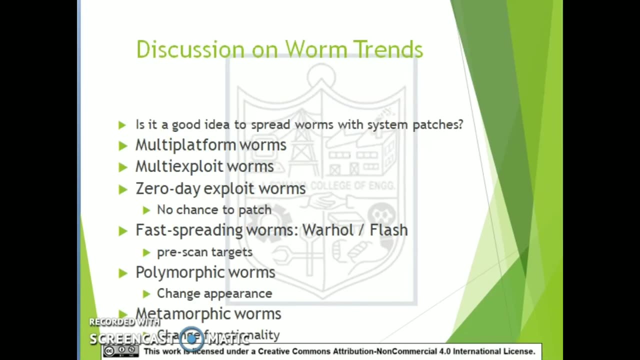 difference between viruses and worms. viruses require interaction, whereas worms act on their own. viruses has to relay on users transferring to infect files or programs, while worms can use a network to replicate itself. speed of worms is more than viruses. discussion on worm trends: it's a good idea to spread worms with system patches. multi-platform worms, multi-expert forms.